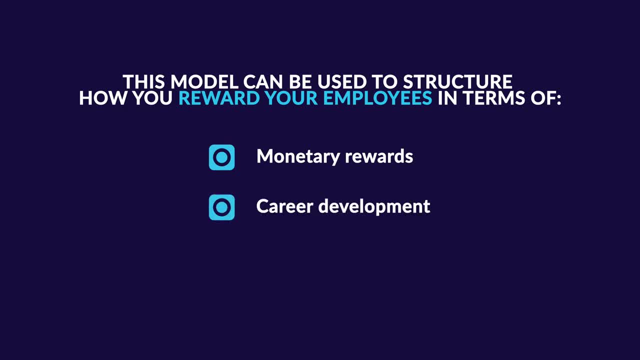 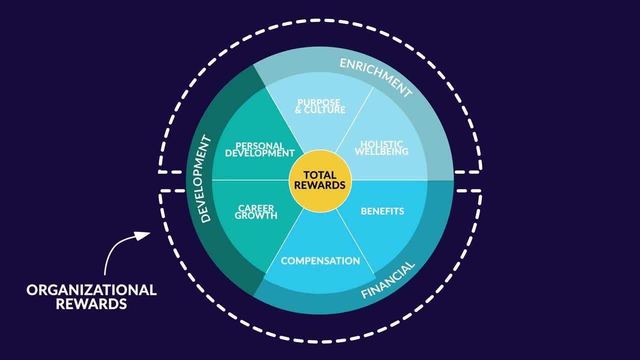 reward your employees in terms of monetary rewards, career development, as well as emotional rewards. As you can see, the model shows organizational rewards, including compensation benefits and career growth. On the flip side, there are individualized rewards, which include personal. 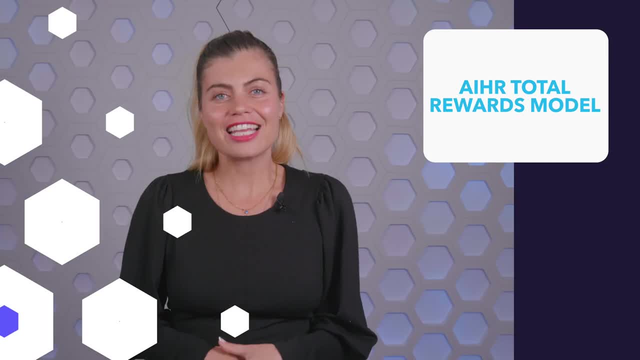 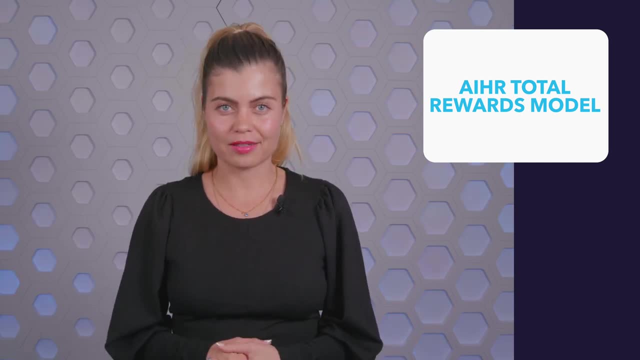 development purpose and culture and holistic well-being. Taken together, they form a unique and differentiated value proposition of the organization for its employees. Let's go over each of these, Starting with compensation- Compensation. Compensation is arguably the best-known way to reward employees and mainly includes salaries. There are two types of compensation, which are base pay and variable pay. Base pay includes hourly wages or salaries. Hourly wages are often given to unskilled, semi-skilled, temporary part-time or contract workers. Employees receiving hourly wages are usually able to earn overtime pay. 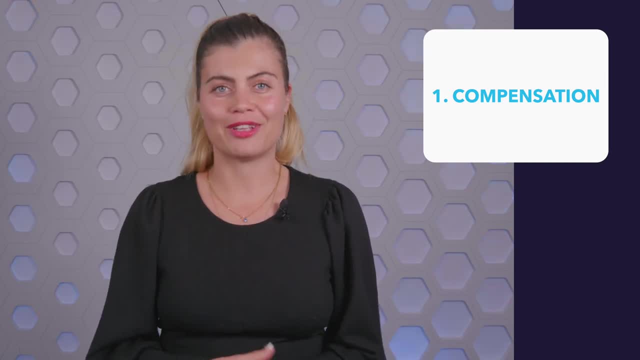 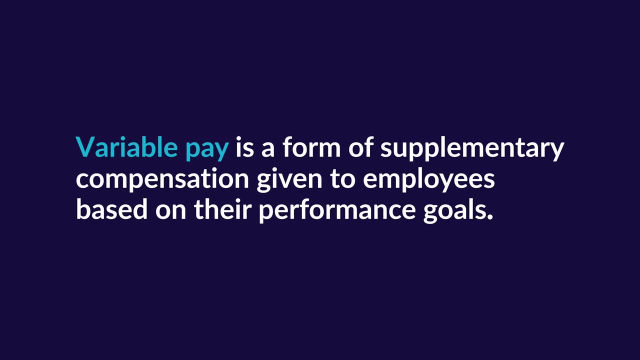 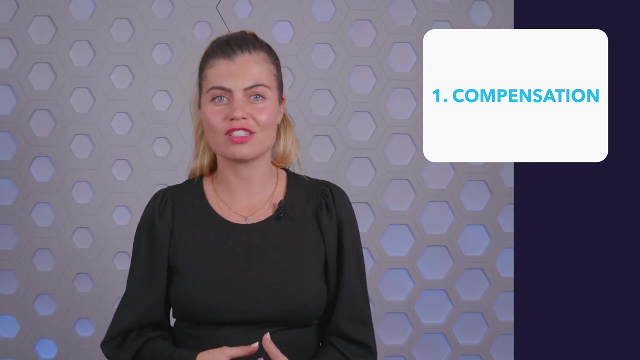 Meanwhile, salaries are typically given to full-time employees. Variable pay is a form of supplementary compensation given to employees based on their performance goals. This can be short-term, which is paid out within one year, or long-term, which is equity billed over time and awarded. 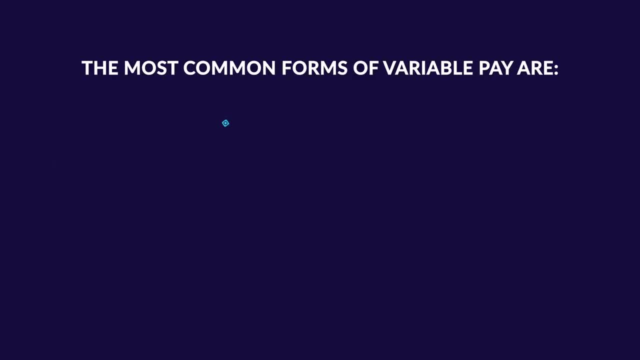 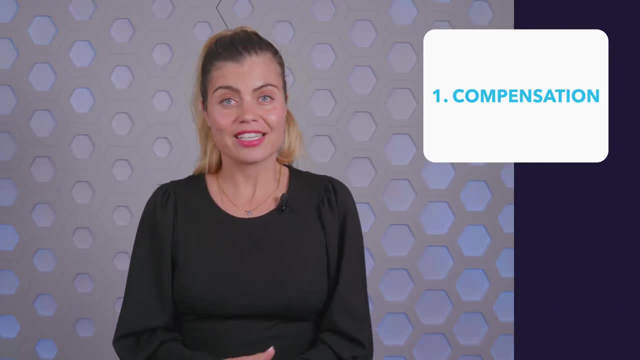 in the future. The most common forms of variable pay are bonuses, sales commissions, referral bonuses or stock options. Compensation plays an important role in maintaining the social contract and is a very important part of the organization. The most common forms of variable pay are bonuses, sales commissions, referral bonuses. 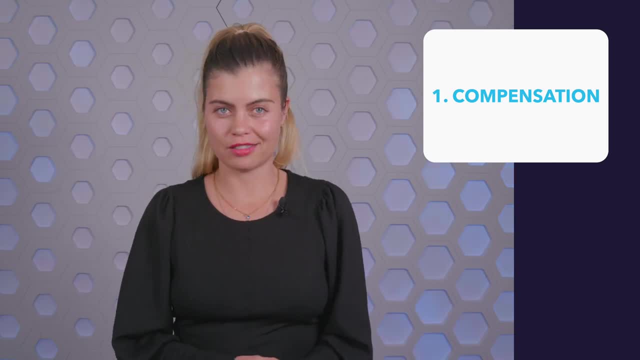 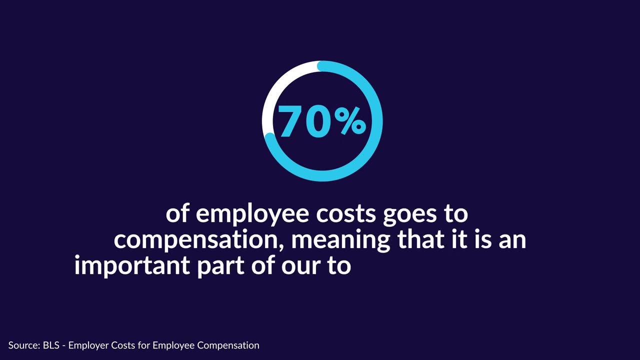 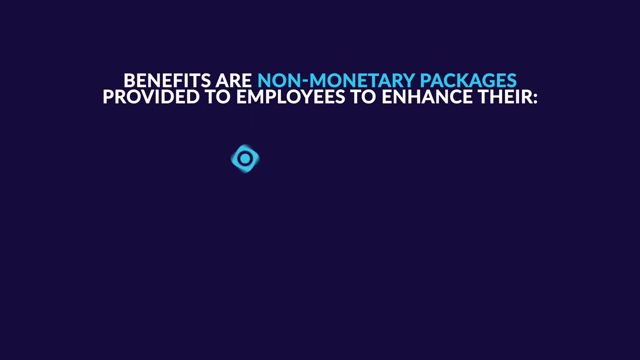 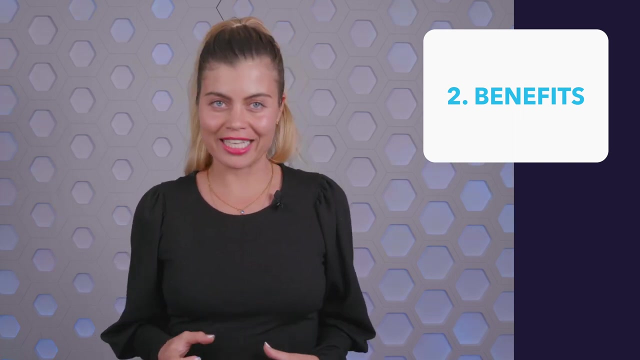 or stock options. Compensation plays an important role in maintaining the social contract and is a very important part of the organization åt. On the employee side, the net gross profit that organizations have with their employees. What's more, 70 percent of employee costs goes to compensation, meaning that it is an 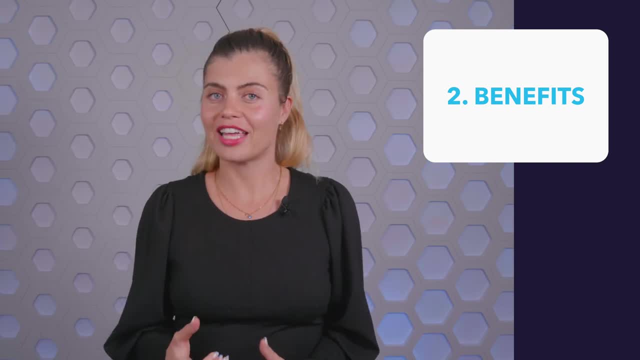 important part of our total rewards model: Benefits. Benefits are non-monetary packages provided to employees to enhance their physical, emotional and familial safety. specific, for example, in the us, health insurance and a 401k pension scheme are common, while in europe, benefits may include additional paternal leave, severance pay or even restaurant vouchers. 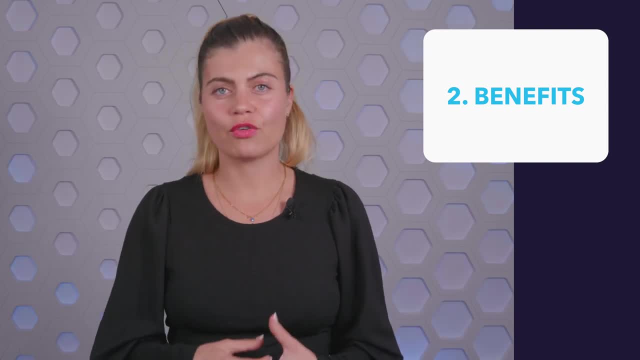 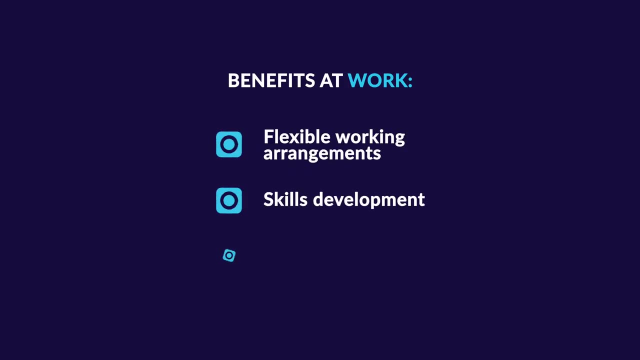 that cover lunch. most benefits fall under one of the four major types of employee benefits, which are: benefits at work, which include flexible working arrangements, skills development and work from home allowances. benefits for health- think of mental and physical health support, including health care, dental care, access to mental wellness apps or company-sponsored therapy. 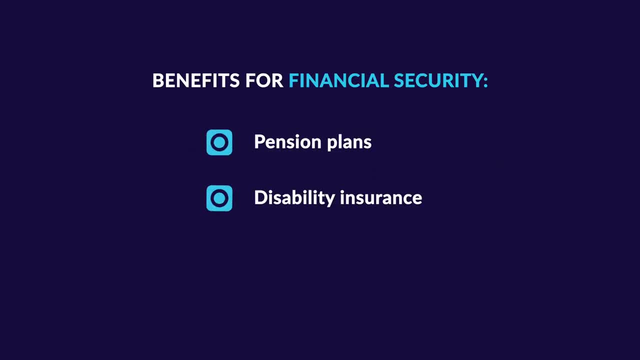 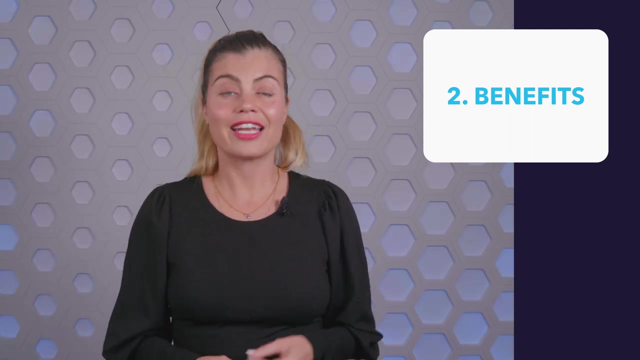 benefits for financial security, which include pension plans, disability insurance or financial literacy programs. lifestyle benefits, which may include a company car, free public transport, but also the ability to work hybrid or remotely, or relocation assistance for international employees or new hires living far away from the office. having a strong employee benefits strategy can help to attract 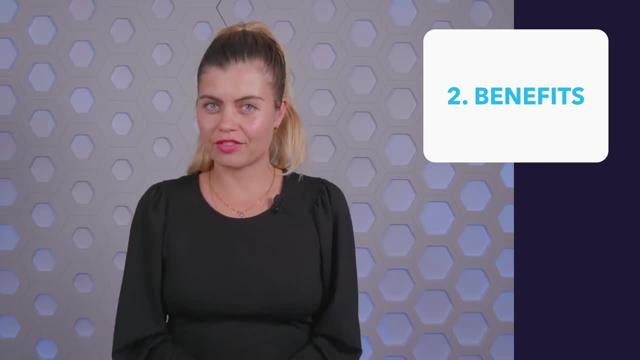 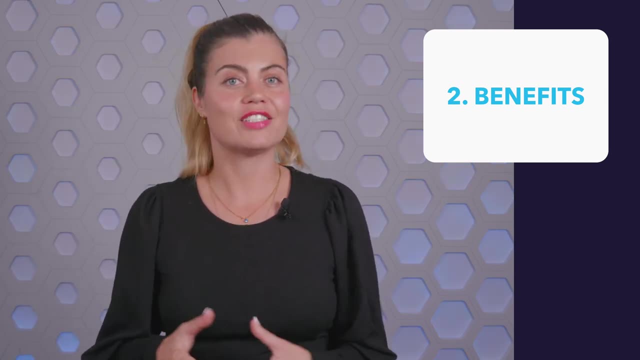 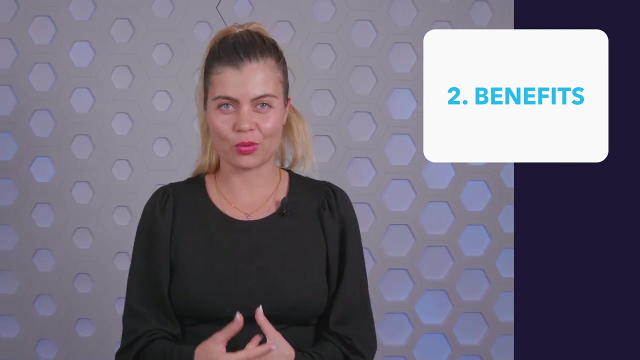 and retain talent and make them happier and more productive. i have seen older employees refuse jobs because they offered little opportunity to build their pensions, and i've seen working moms switch jobs because their company didn't offer flexibility in working hours. benefits are a great way to differentiate yourself from other organizations. career growth- this aspect of 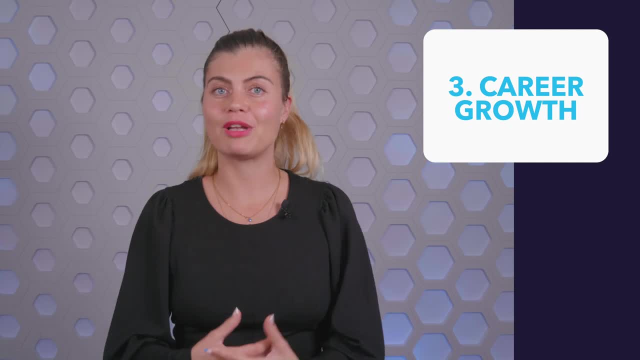 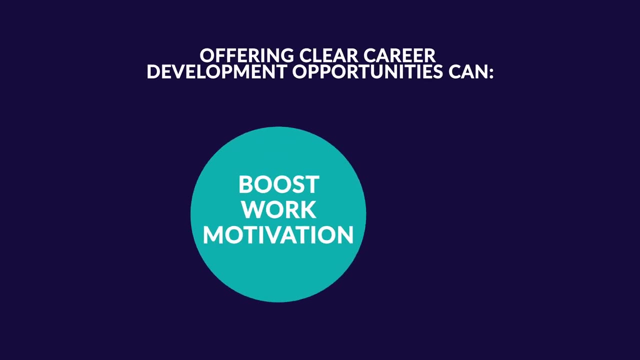 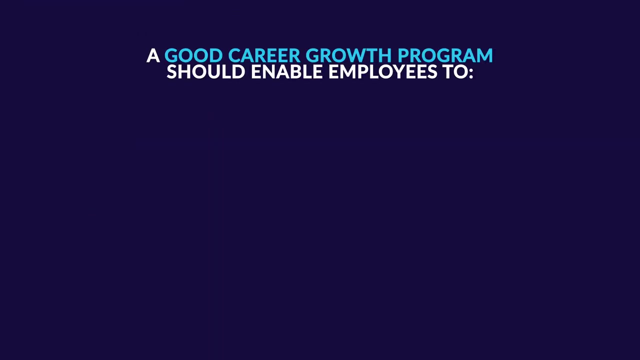 a Total Rewards Model focuses on whether companies enable employees to advance in their career path. Offering clear career development opportunities can boost work motivation, reduce unwanted turnover and help employees avoid burnout. A good career growth program should enable employees to gain and enhance their capabilities, excel in their current and future roles, work towards promotion. 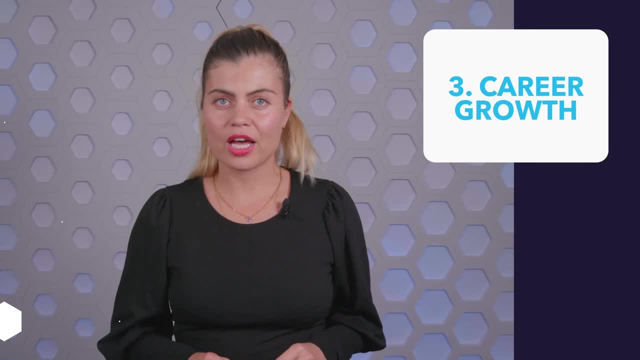 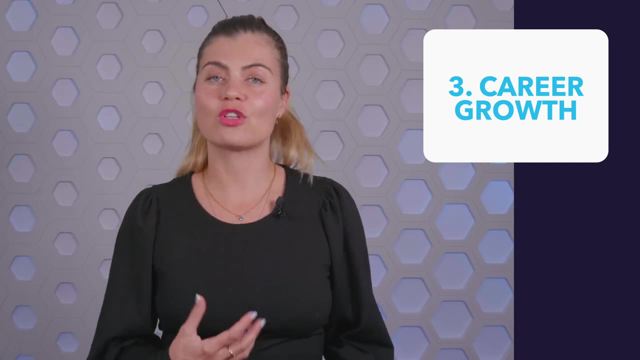 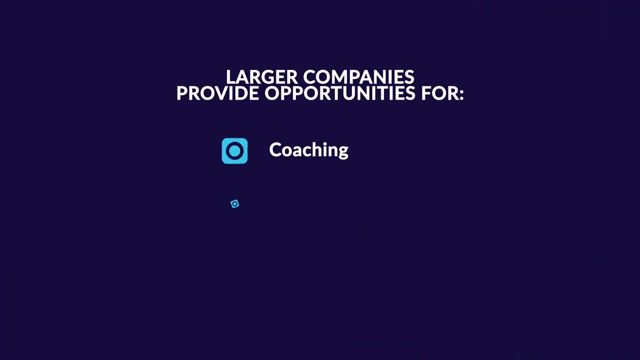 opportunities in more senior positions. This is an area where companies can set themselves apart. Larger companies are able to provide more complex career paths, either through specialization or promotion to more senior leadership positions. This includes opportunities for coaching, mentorship or challenging work assignments. On the other hand, smaller companies offer 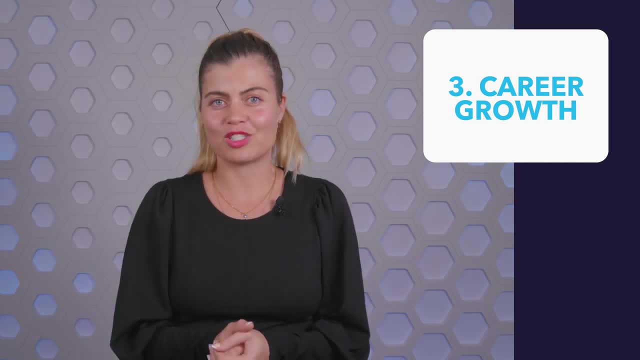 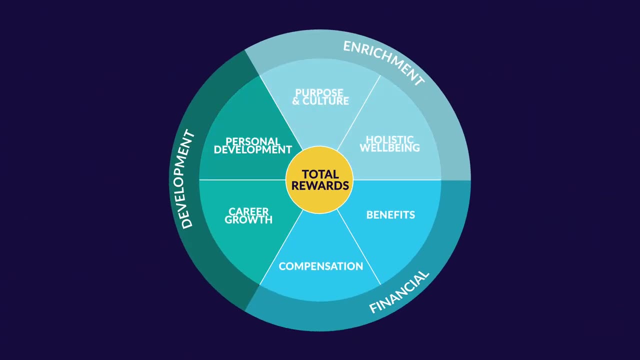 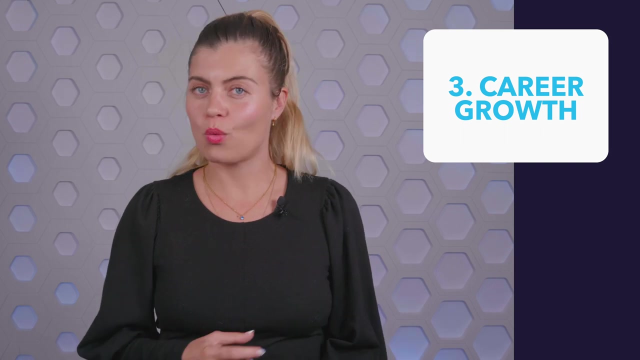 employees broader roles in which they get a lot of different responsibilities and manage end-to-end processes. Taken together, career growth, compensation and benefits form the enablers in our Total Rewards Model. They are the prime reason why people work, and without these three work will not happen. 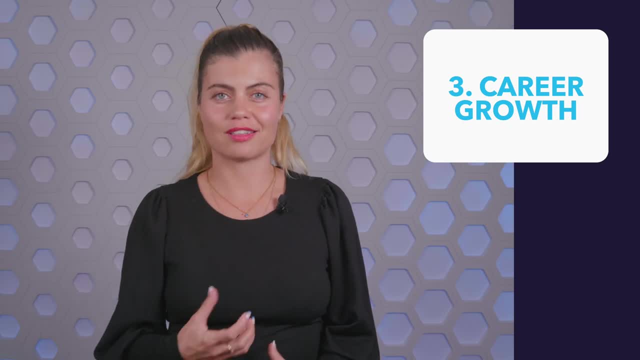 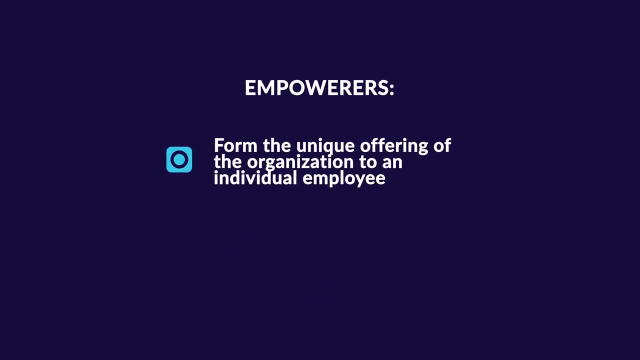 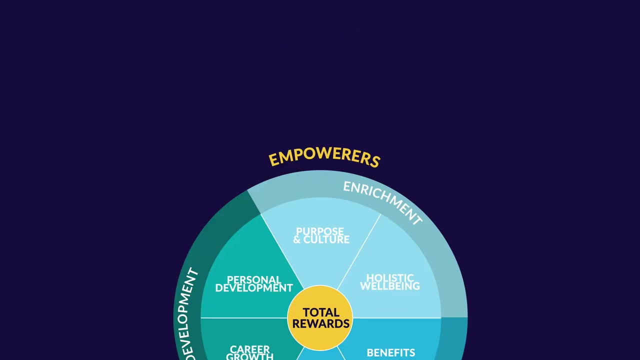 Once the enablers are taken care of, the empowerers come into play. On the flip side of the model are the empowers. These form the unique offering of the organization to an employee. They differentiate the organization's employee value proposition from its competition. These are personal development, purpose and culture, and holistic. 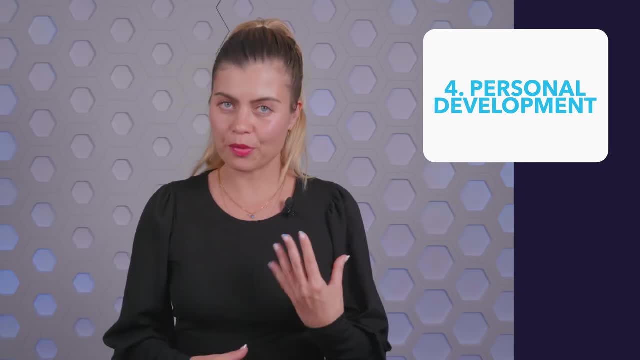 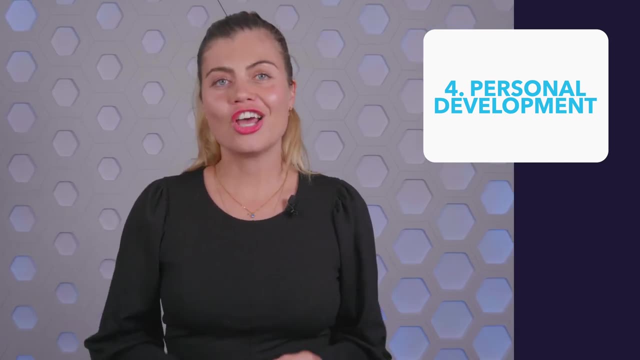 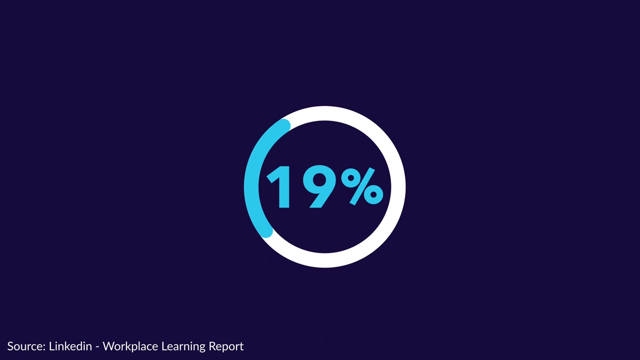 well-being. Personal development- The ability to promote Ability to grow personally and professionally- is another key consideration when people decide where they want to work. Learning new skills is crucial to developing yourself and remaining relevant in your career. According to LinkedIn, 94% of employees would stay at a company longer if it invested in. 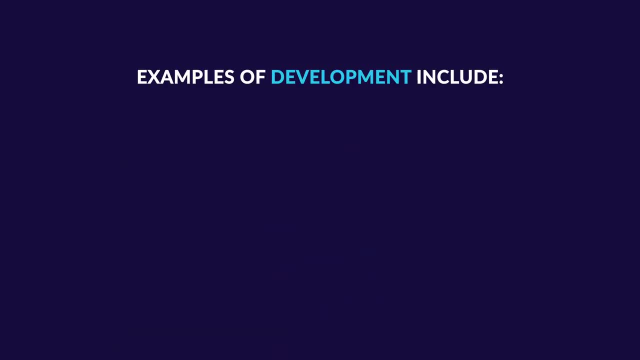 their development. Examples of development include personal learning allowances. Often times, employees get a budget for learning, which is sometimes included in the job offer. The ability to learn new skills through either the company's formal training programs or through challenging assignments, Career training and mentoring programs. 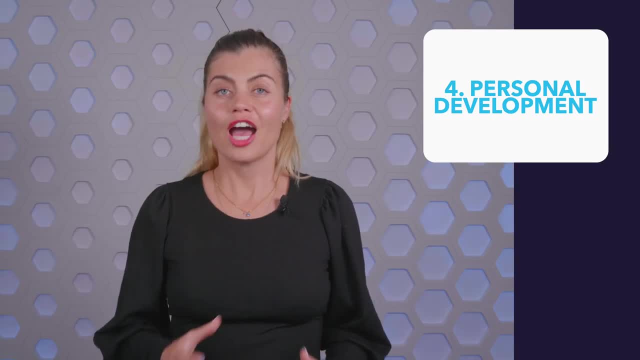 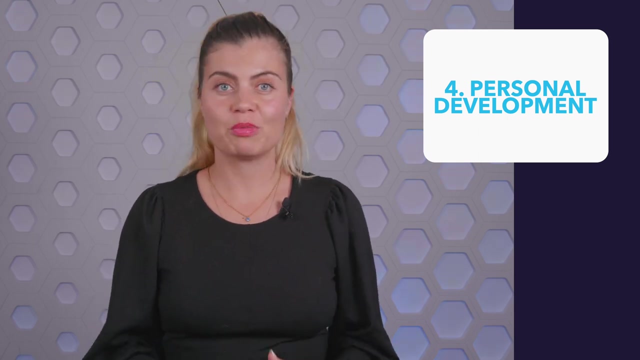 Leadership development plans, Personal development and career growth complement one another. Sometimes they are fully aligned, but sometimes people are looking to develop themselves outside of the organization. I know someone who wants to become an entrepreneur. I know someone who wanted to work less to have more time- to be a football trainer for. 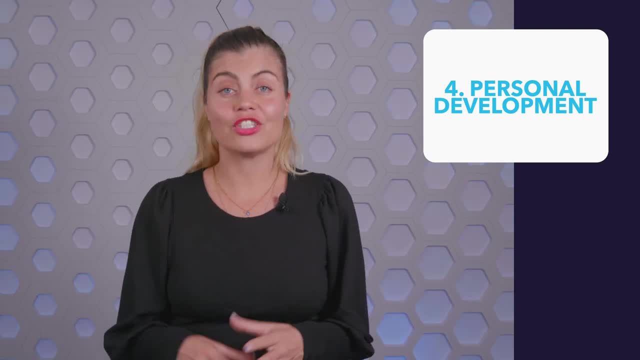 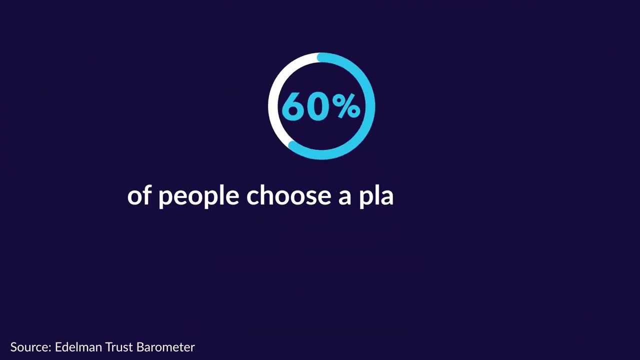 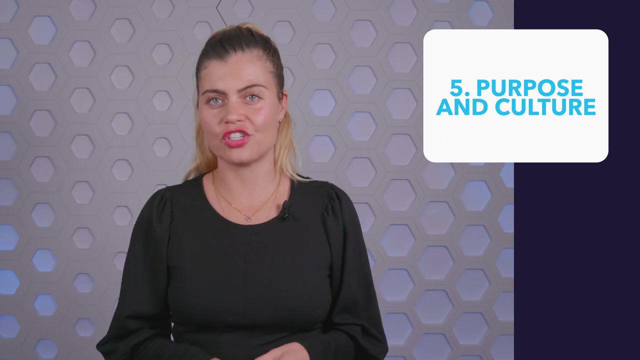 his son's team That flexibility is also part of the unique value that an organization can offer an employee Purpose and culture. 60% of people choose a place to work based on their beliefs and values. This makes connecting employees' purpose with the purpose of the organization more. 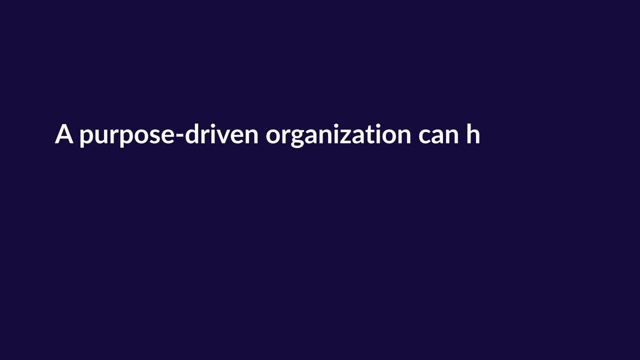 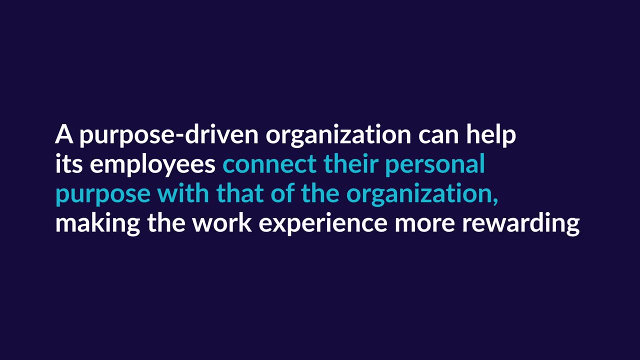 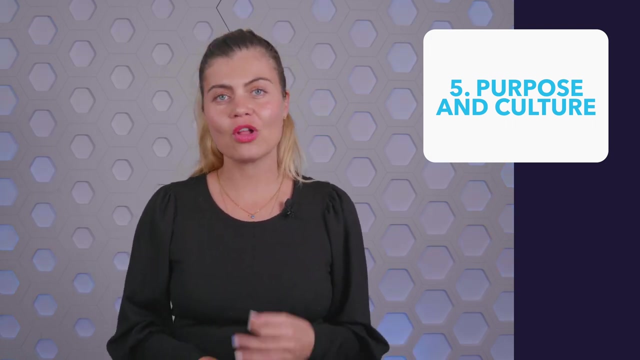 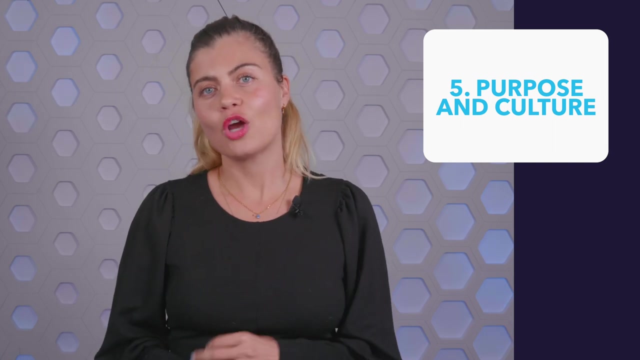 important than ever. A purpose-driven organization can help its employees connect their personal purpose with that purpose. This makes the work experience more rewarding. Beyond organizational purpose, employees also place more value on finding a company with a suitable internal culture. Some people might do well in a more performance-driven market culture, while others would thrive. 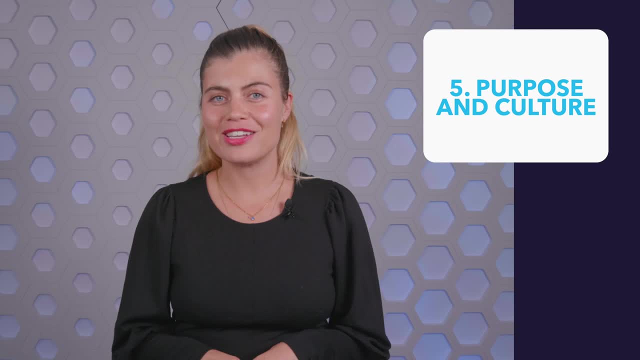 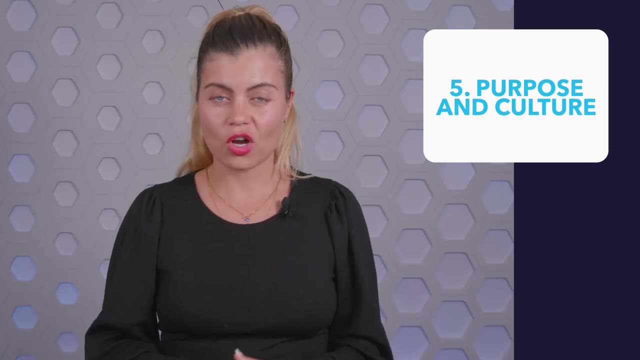 in a more collaboration-driven clan culture. For more information about organizational culture, check out our full explainer video here. Workplace culture also includes the way everyone works. Workplace culture also includes the way everyone works, The way employees are recognized by their manager or peers, and whether the organization 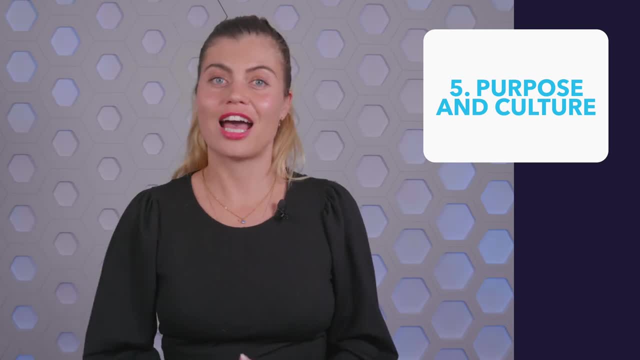 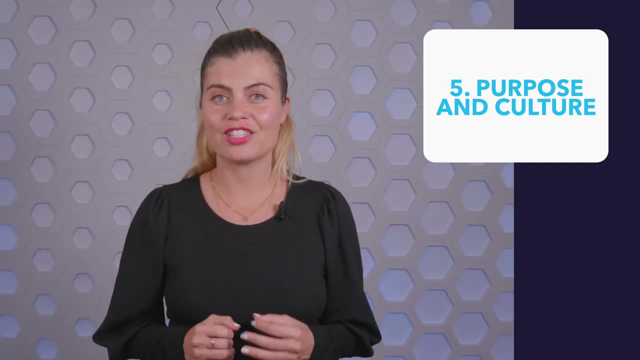 works on diversity, equity, inclusion and belonging. Purpose and culture form the flipside of compensation. Oftentimes you see organizations with a strong purpose compensate less. For many, the main reason to work there is the impact they make, not the money they earn. 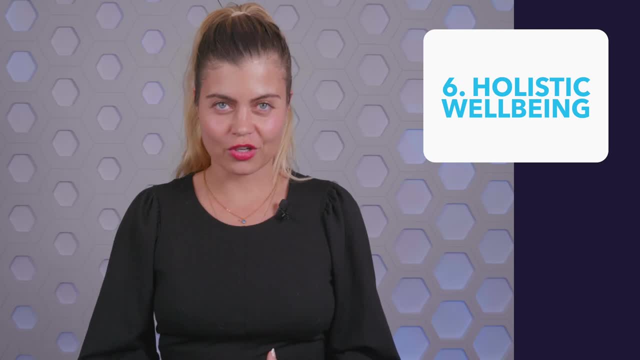 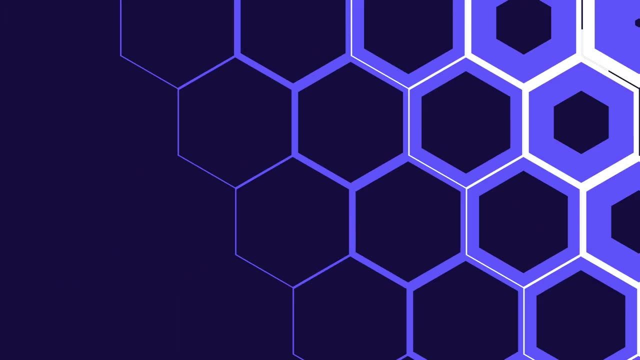 Holistic well-being. Well-being is becoming increasingly critical to attracting and retaining employees. Well-being is becoming increasingly critical to attracting and retaining employees- employees- and ensuring that they are engaged, motivated and productive. According to Champion Health, one in five employees cites poor mental. 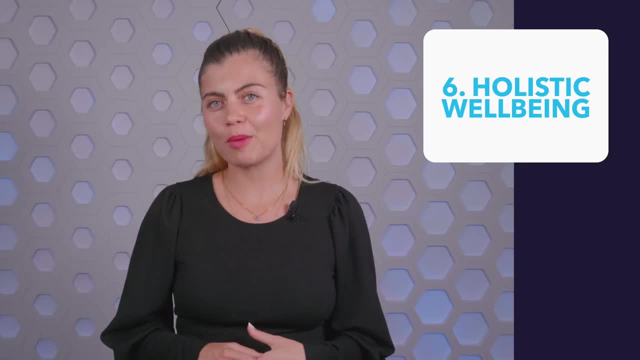 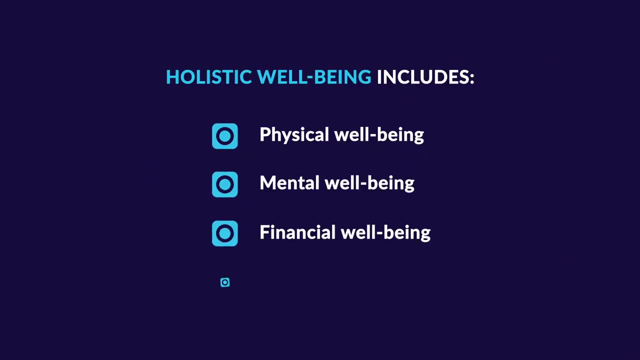 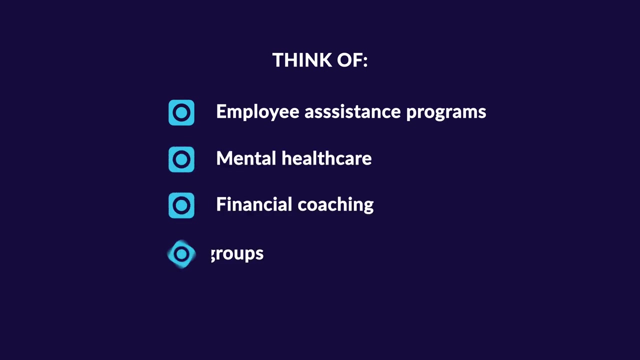 health as a factor that affects their productivity. Holistic well-being is also a way for employers to set themselves apart. It includes physical, mental, financial and social well-being. Think of employee assistance programs, as well as access to mental health care, financial coaching, employee resource groups and other wellness programs. 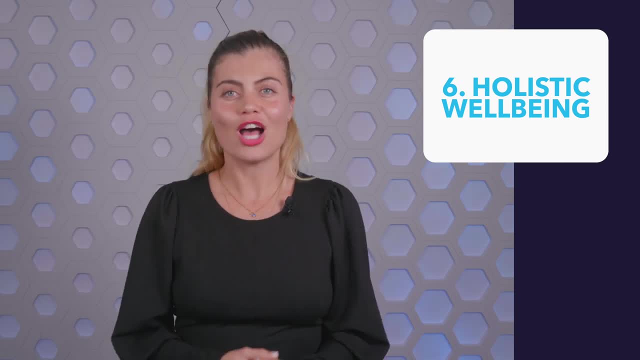 Having a healthy and inclusive work culture is crucial to supporting your employees well-being. This can mean ensuring that your employees have ample time off to unwind. Holistic well-being is an extension of benefits. Many of the initiatives to increase well-being are different forms of benefits. 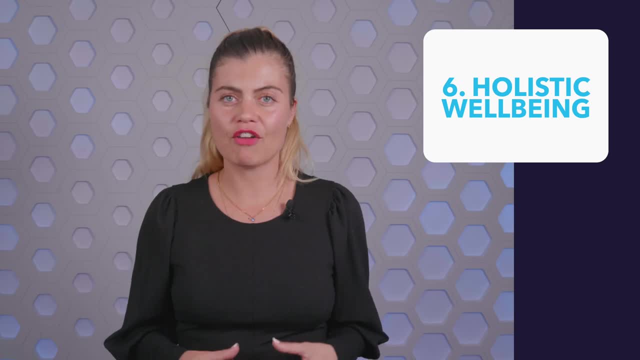 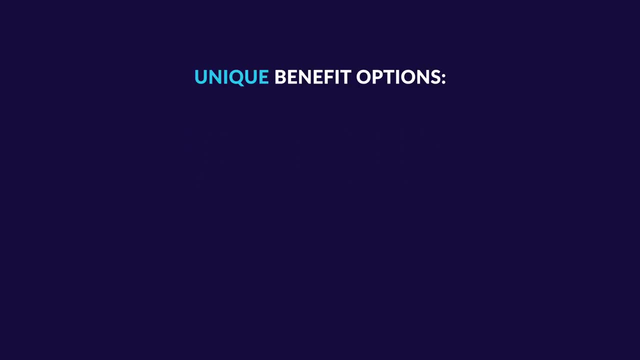 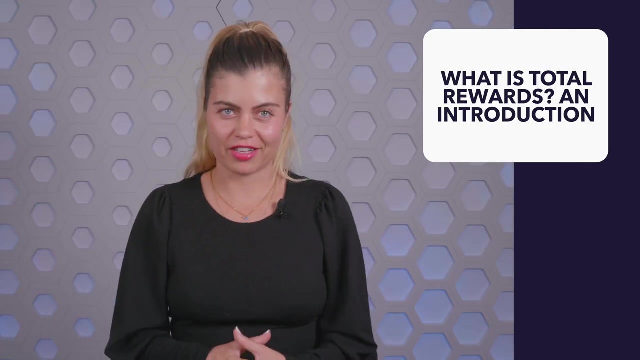 Examples include giving extra days off or even offering a four day work week. Menstrual leave is also becoming more popular. You can even consider more unique benefit options, such as birthday leave, bringing your pet to work day or on-site massages. These are some of our favorite benefits. 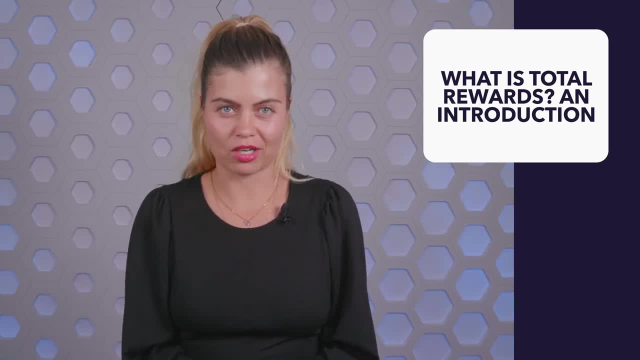 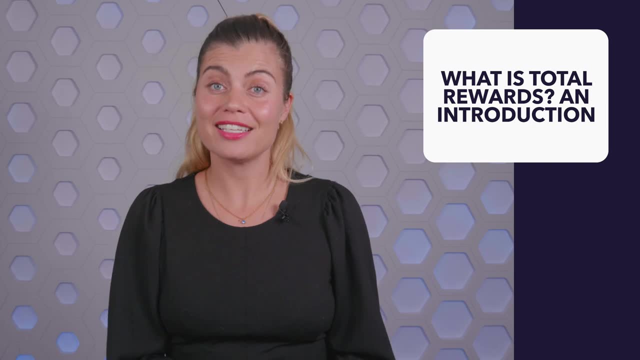 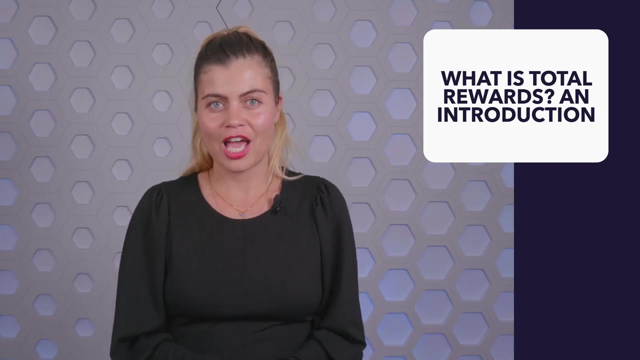 A few that we haven't mentioned yet are flexible working policies so employees can take care of elderly relatives, or volunteers time off, where employees get paid time off to do volunteer work. Both of these contribute to an organization's unique culture and purpose. They can also create a unique total rewards offering for their employees. 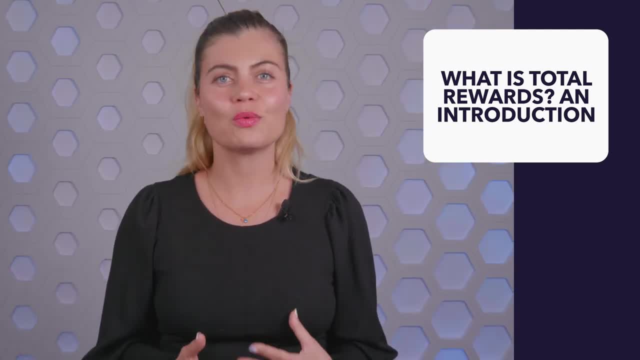 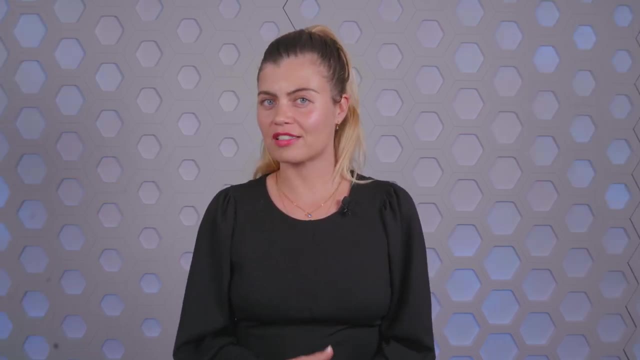 This is a great way to create a unique total rewards offering for your organization. It's so important to attract, retain and motivate employees. And there you have it: The six elements of a successful total rewards strategy, along with examples of programs that you can implement in your organization. 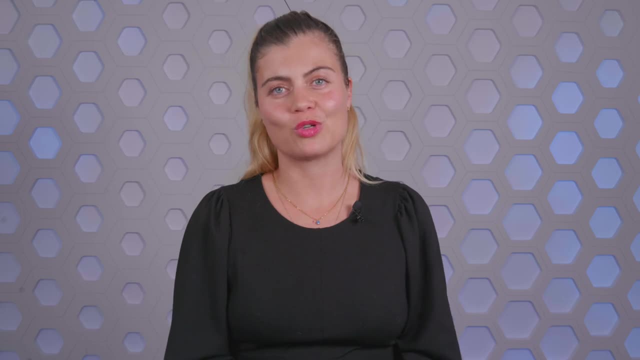 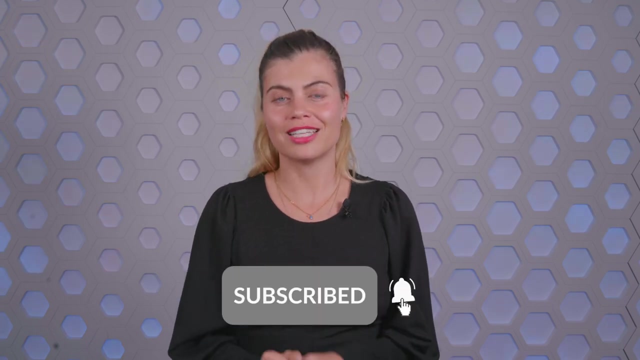 Do you have more examples of things to include in a total rewards model? Let us know in the comments down below. And don't forget to like this video, subscribe to our channel and hit the notification button. Bye.